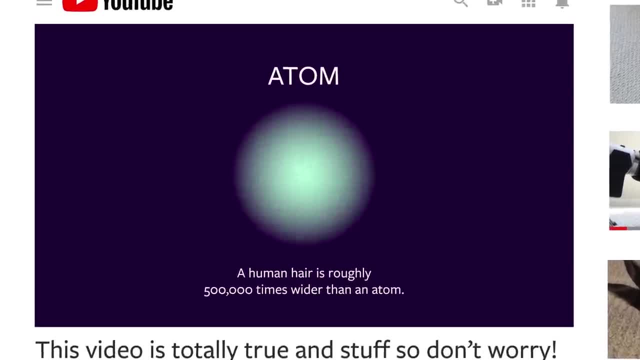 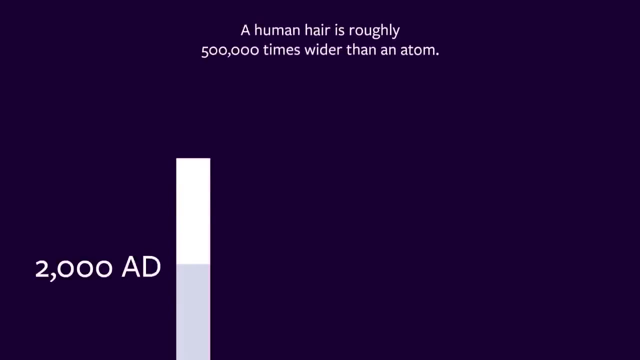 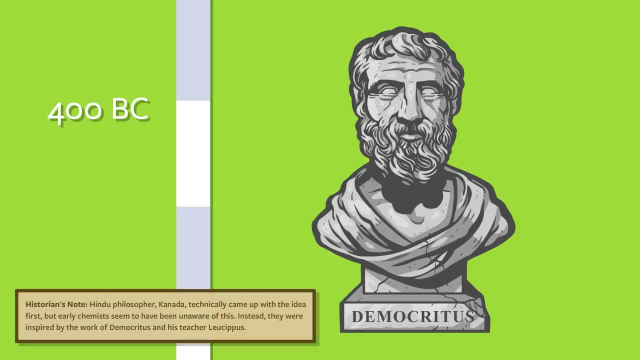 No, Now you are extra curious. You want to know for yourself exactly why it is that scientists think they know that atoms exist. Well, to find out, we must travel back in time to ancient Greece. Meet Democritus, the man that many historians credit for first clearly proposing the idea of an atom. 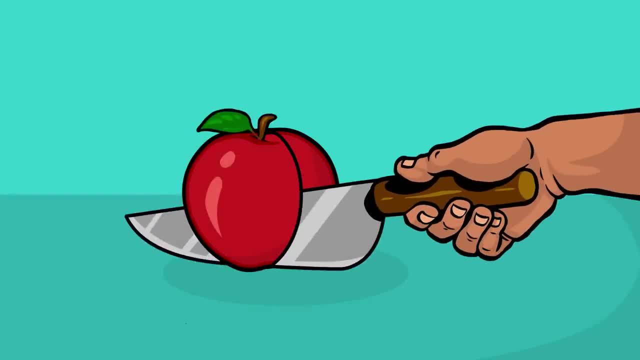 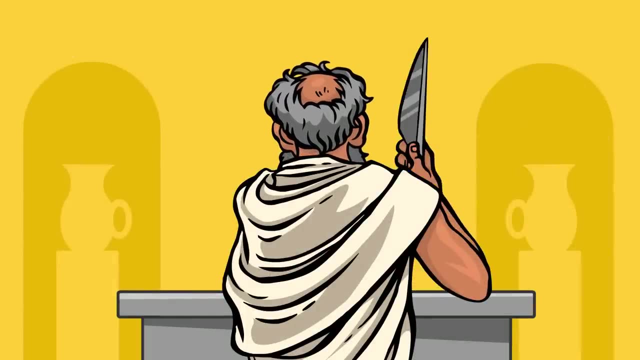 In his day, it was thought by some that if you were to chop up a piece of matter, an apple for instance- you could just keep on chopping forever and ever. there was no end to smallness, For reasons not fully agreed upon by historians. 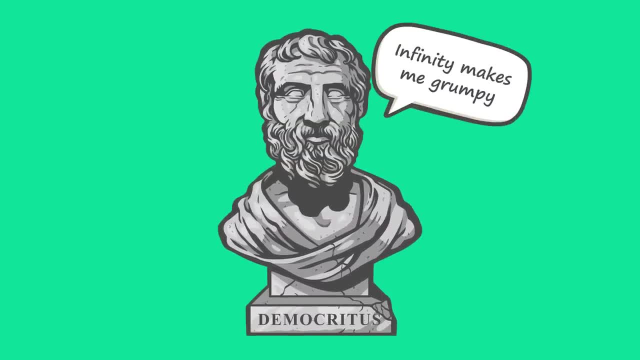 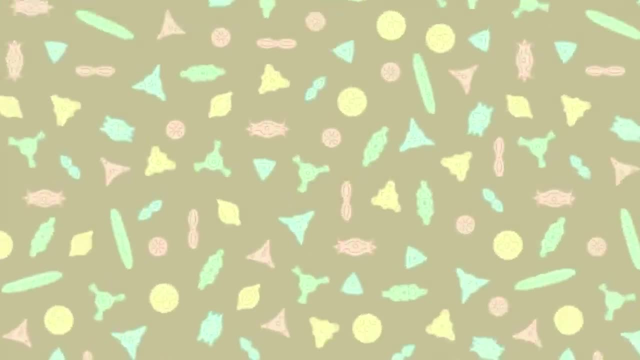 this concept did not sit well with Democritus. Instead, he insisted that at some point you would reach particles so small and so indestructible they could not be divided any further. He called them Atomos, or atoms, which means uncuttable. 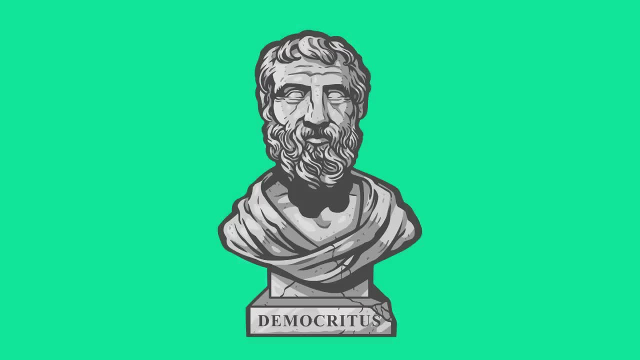 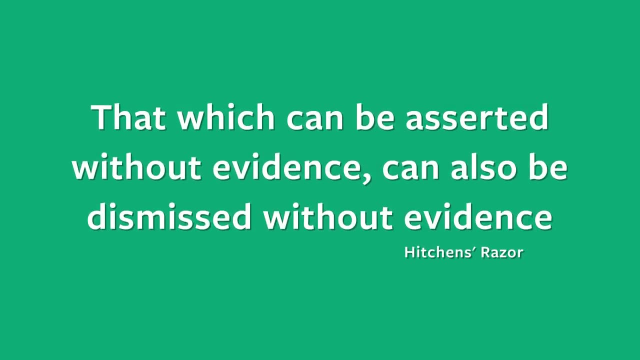 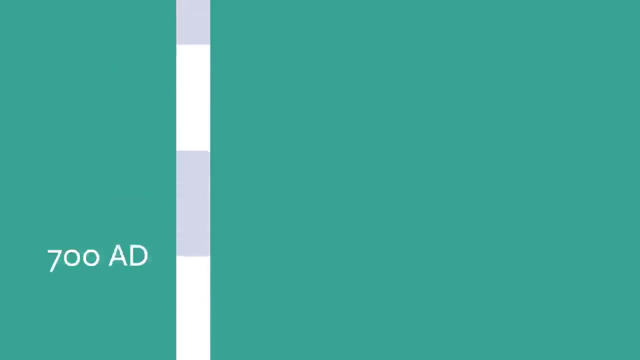 Now, Democritus didn't actually have any evidence to back up his claim, and because of that, many people simply rejected it. After all, that which can be asserted without evidence can also be dismissed without evidence. Let's fast-forward several hundred years and hop on over to the Arabic world. 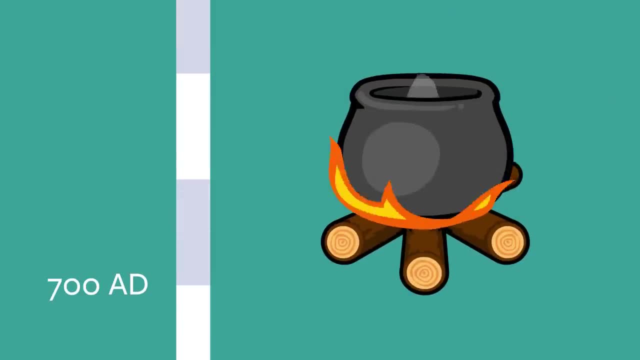 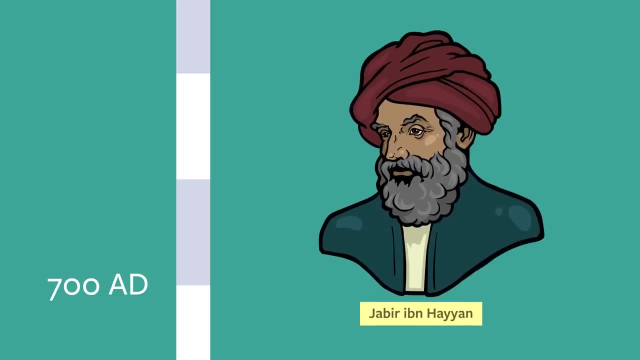 You probably know that salt can be extracted from seawater by simply letting it evaporate or boiling it dry. People have been doing this forever, but alchemist Jabir ibn Hayyan and those that followed his work took the science of extraction to a whole new level. 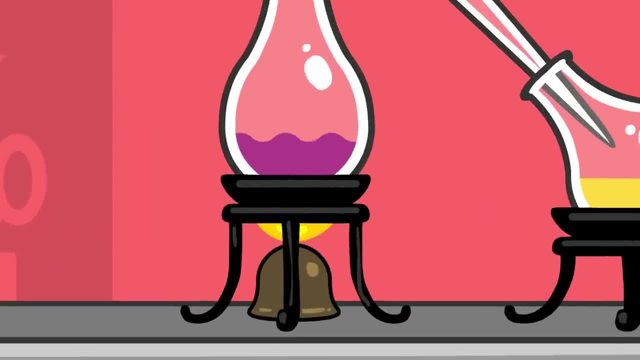 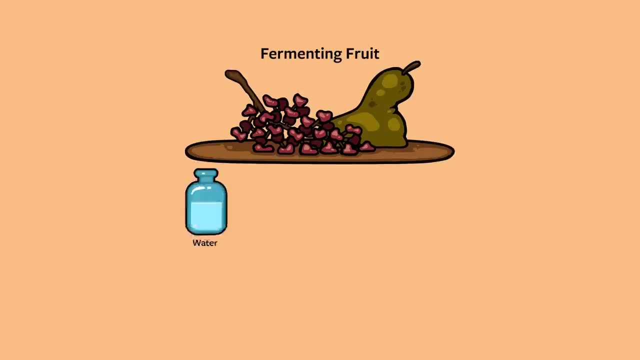 Through careful experimentation, they developed complex processes of filtration, boiling, vapor collection and cooling. They found that crude starting materials could be divided into multiple incredibly pure substances. Pure meaning they appeared to be consistent all the way through, unlike the complex mixtures of matter often found in nature. 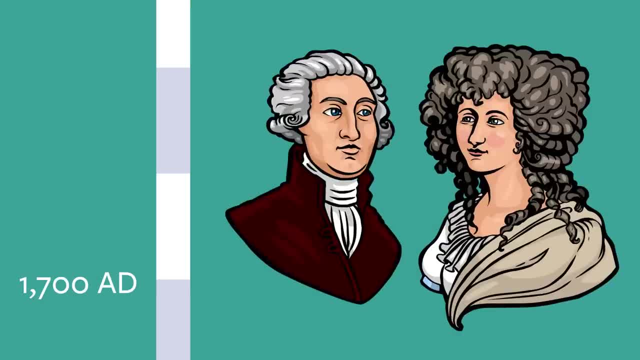 In the 1700s, a French husband-and-wife scientific duo, Marianne Poults and Antoine Lavoisier, studied and built upon the work of their Arabic predecessors. They found that certain pure substances could be broken down even further through chemical reactions. 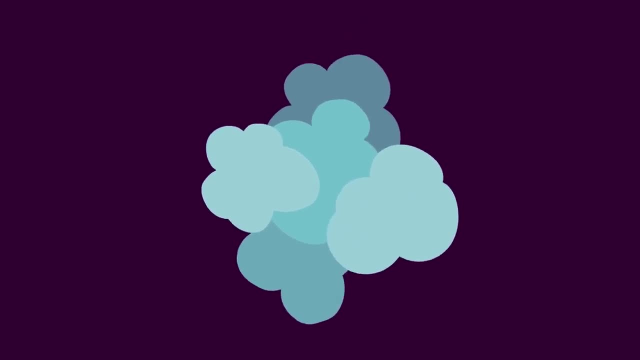 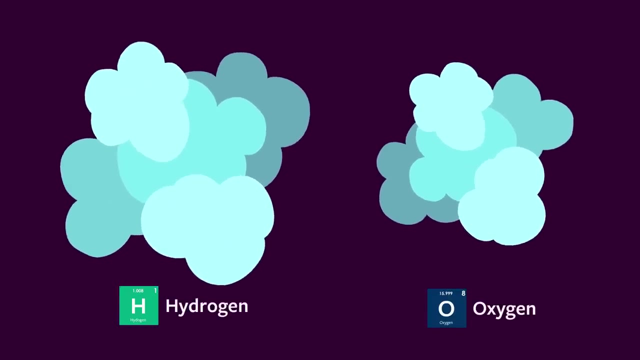 Water, for example, can be boiled into steam, which is still water, but it can also be split into two pure gases: hydrogen and oxygen. No matter how hard the couple tried, however, they could not reduce oxygen or hydrogen into simpler gases. 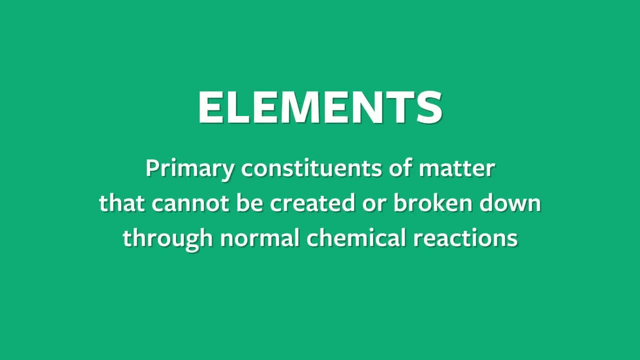 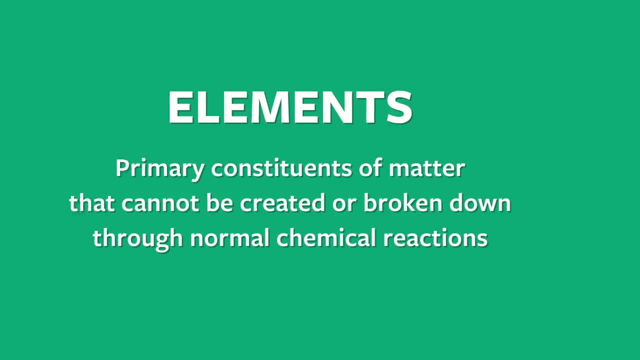 They concluded that the gases must be elements, foundational substances that cannot be created by the use of chemical reactions. They were created by mixing other chemicals together and cannot be broken down any further. With this concept in mind, scientists everywhere began searching for and listing as many elements as they could. 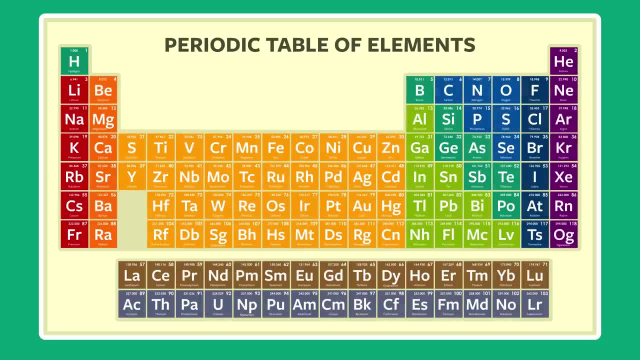 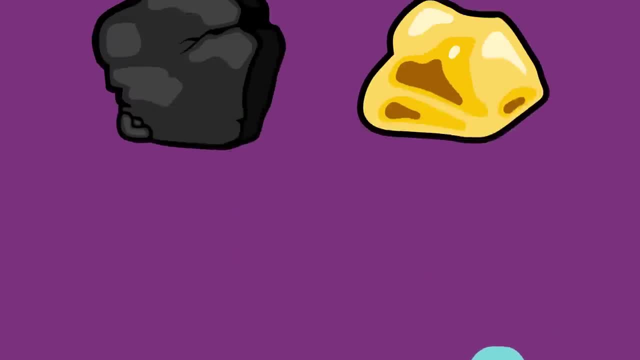 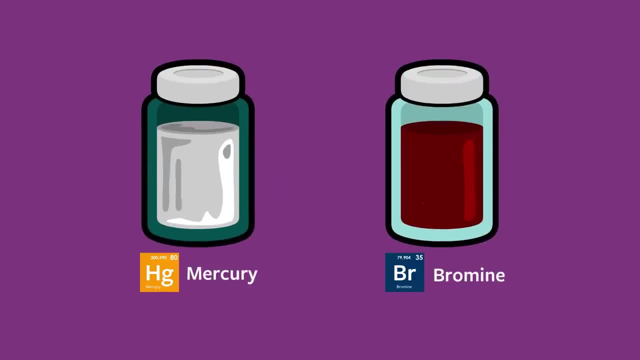 eventually discovering all 118 listed on the modern periodic table. Some, such as oxygen and hydrogen, are gases at room temperature. Others are solids, such as elemental carbon and gold. Others still are liquid at room temperature: mercury and bromine. It was also found that, under the right conditions, 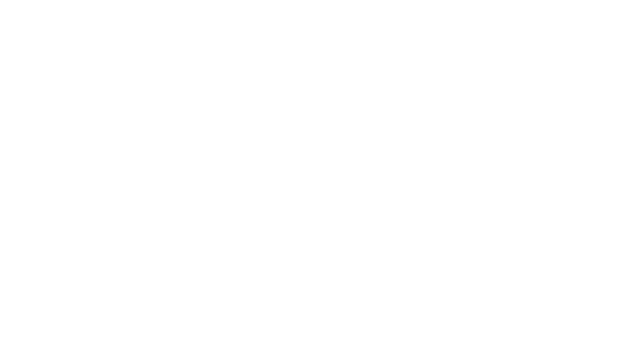 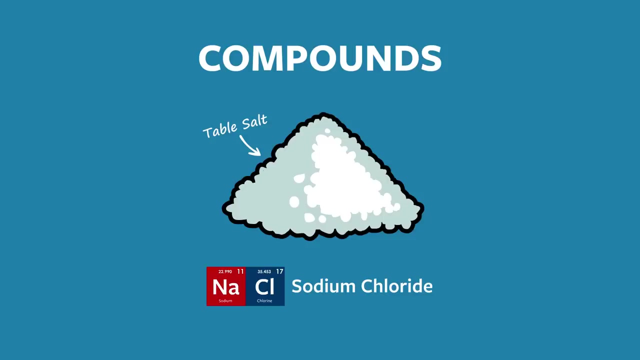 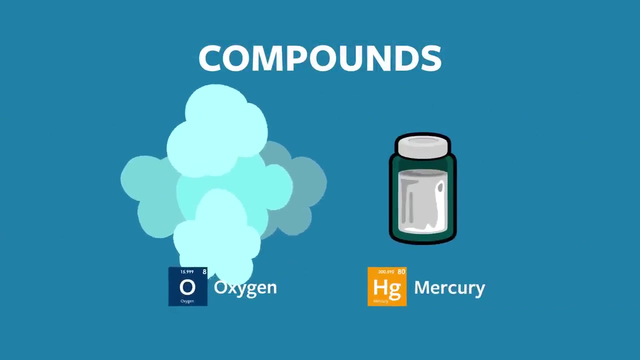 pressure and temperature. certain elements will react with each other upon mixing to form new substances with new properties. These are called compounds. The elements oxygen and iron can react to form a brown powder known as rust. Oxygen and mercury react to form a toxic orange powder. 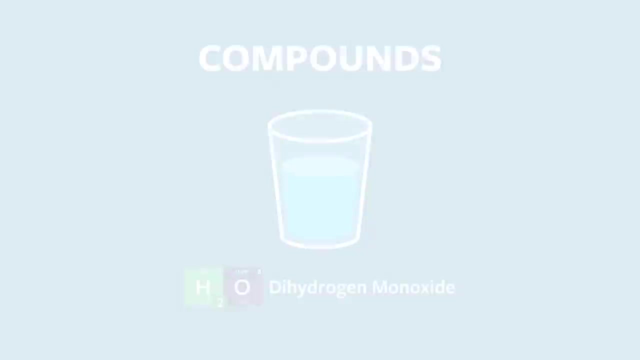 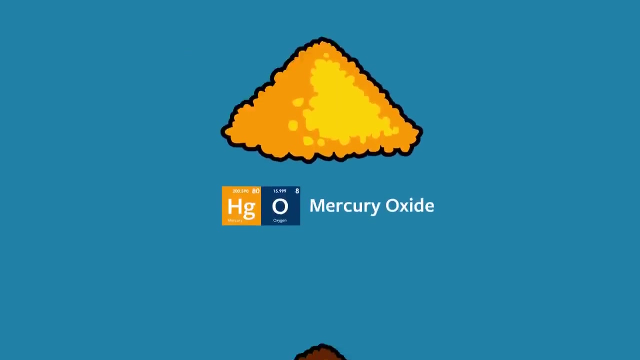 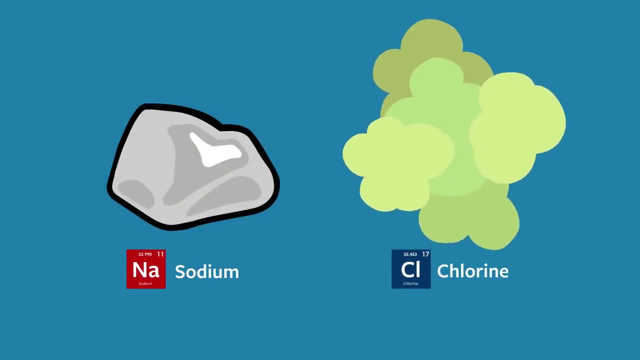 Oxygen and hydrogen react to form a clear, refreshing liquid. You probably know it as water Water. Though the steps may be complicated, all of these reactions can be reversed. Elements can be re-separated and the amount of each element we get back after separation. 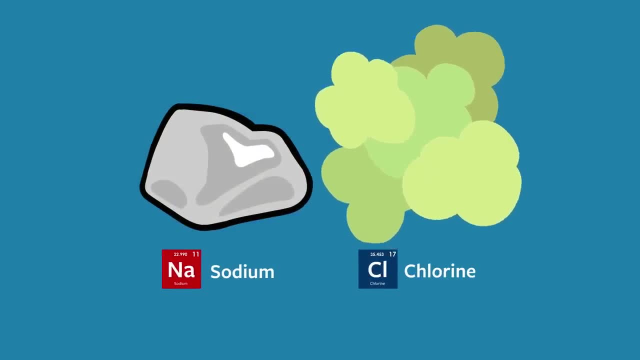 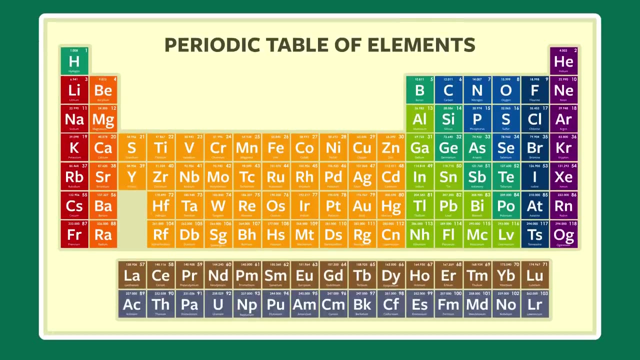 is always exactly equal to the amount that had reacted to form the compound in the first place. Wonderful Elements are real and they appear to be essentially indestructible, but what are they made of? If you were to zoom in on one, 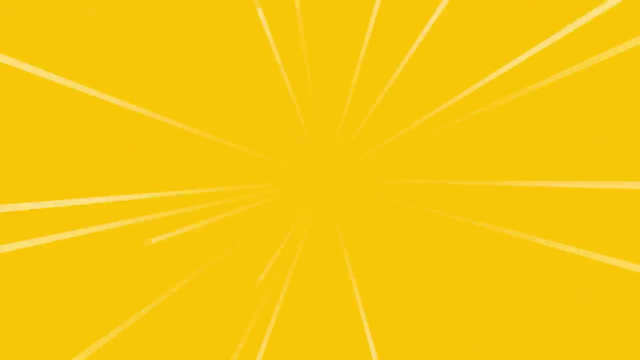 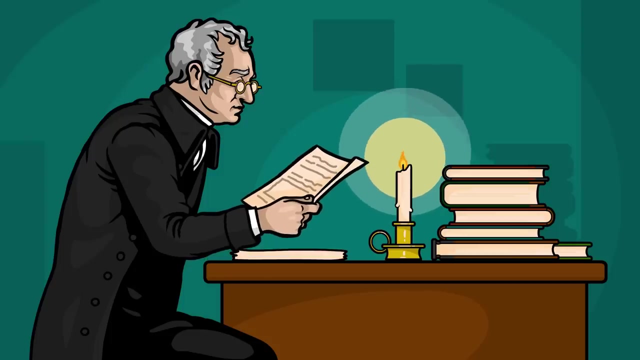 a chunk of pure gold, for example? can you just keep zooming in forever and ever, saying nothing but pure gold for infinity? In the early 1800s, a school teacher from England named John Dalton grew fascinated with chemistry, Along with conducting several experiments of his own. 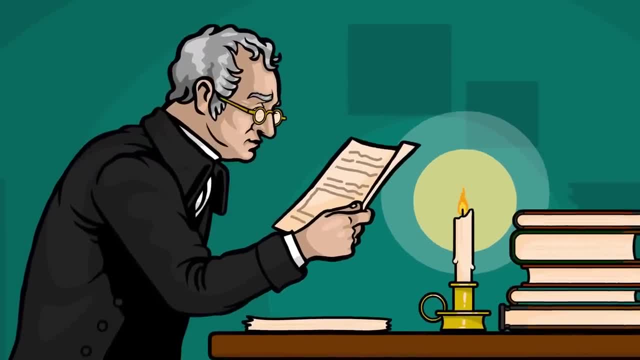 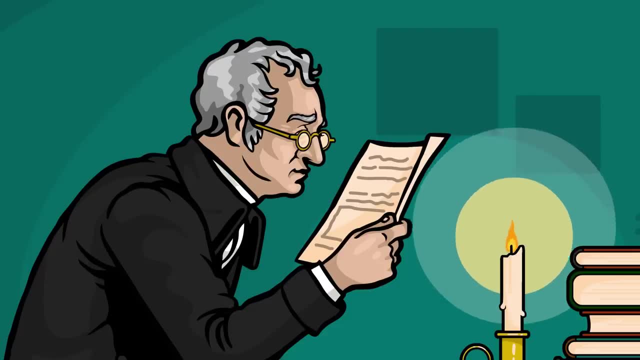 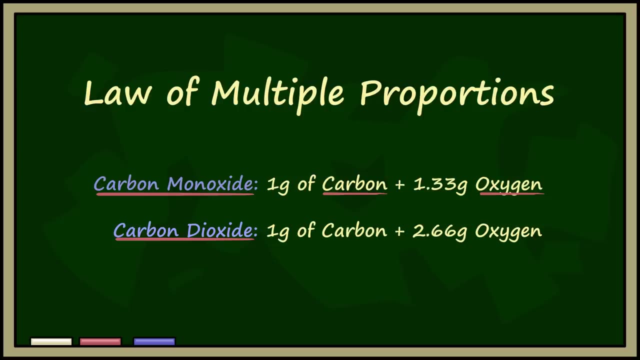 he read about every experiment he possibly could, paying special attention to the quantities of each element used up in every chemical reaction. In these numbers, he was surprised to find a pattern emerge. When two elements can react to form multiple types of compounds, they always do so in small whole-number ratios. 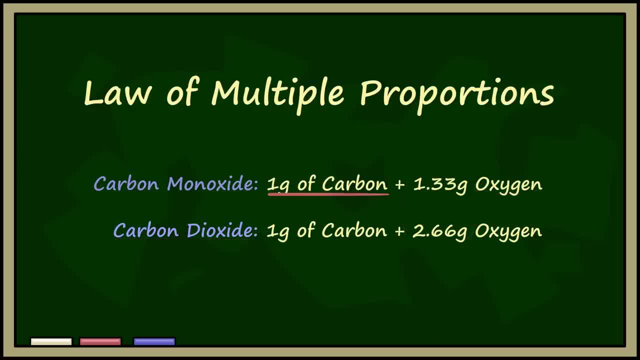 In this example here we see that in order to transform a gram of carbon into pure carbon monoxide, we need to add 1.33 grams of oxygen. To turn a gram of carbon into pure carbon dioxide, we need to add exactly twice as much oxygen. 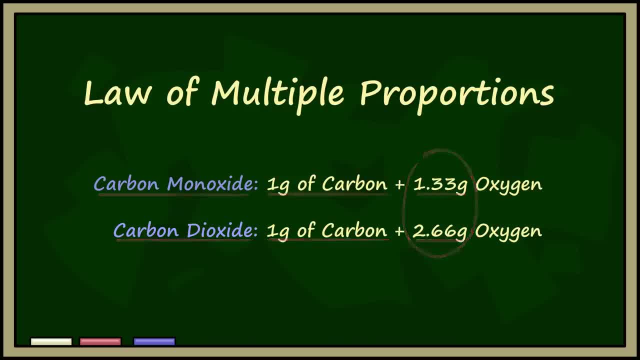 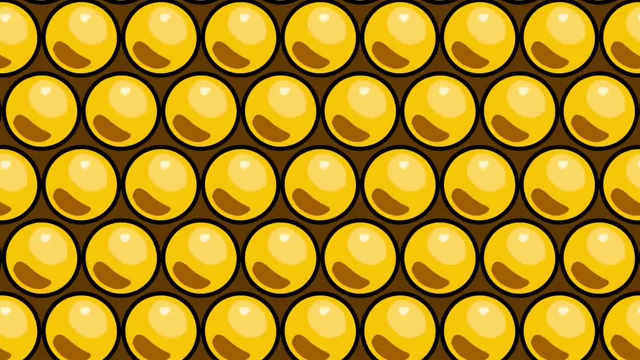 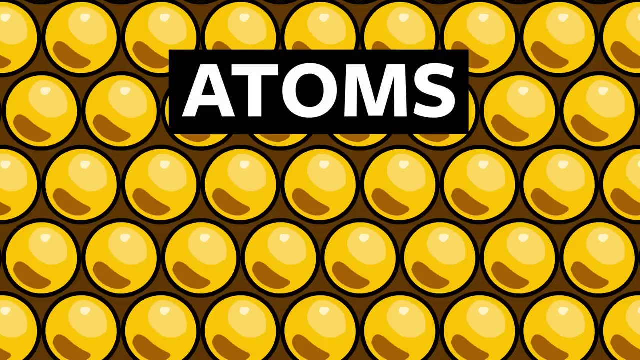 That's 2.66 grams. This and many other similar observations strongly suggest that oxygen and other elements are made of tiny, indivisible units: Atoms. He didn't know exactly how small an atom was, but the numbers suggested that the atoms of a single element. 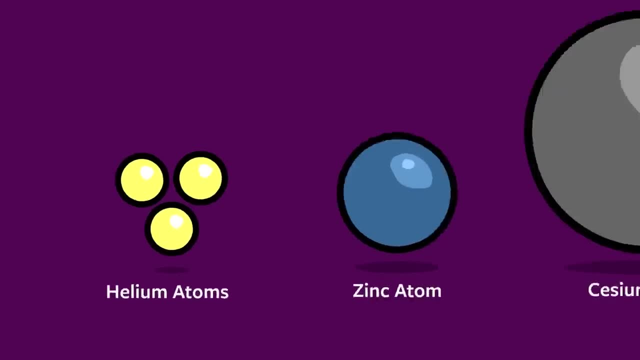 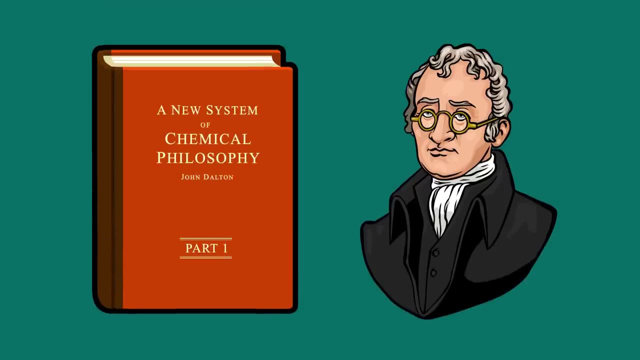 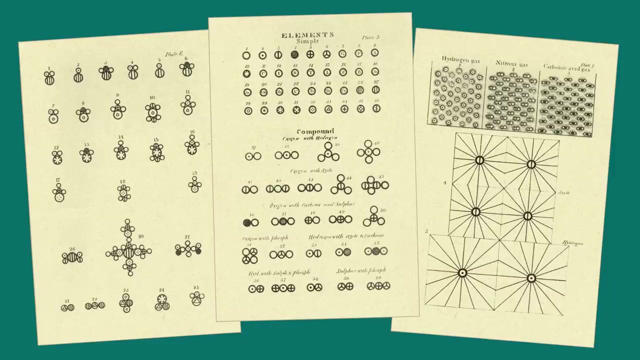 were all nearly identical in size to each other, but different in size to the atoms found in other elements. In 1808, he wrote a 560-page book that briefly mentioned his discovery. It even came with some quite beautiful drawings. While scientists weren't fully convinced that atoms were real, 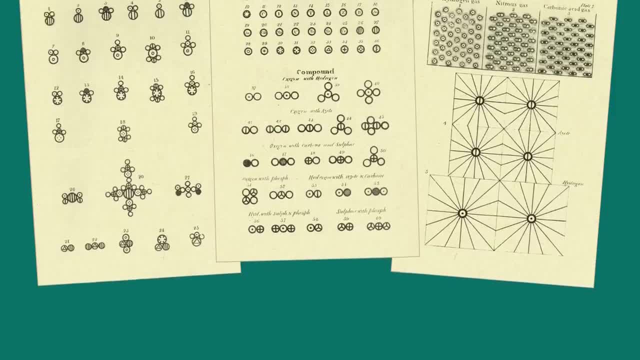 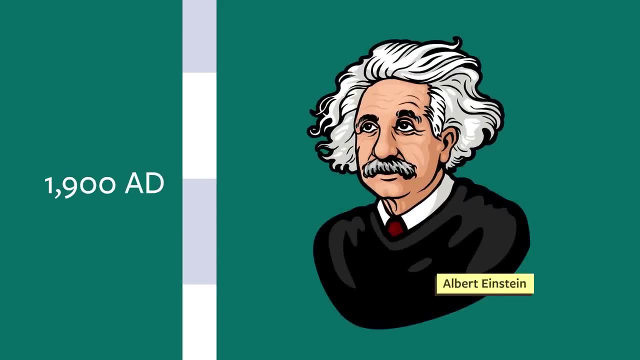 they did find the concept of atoms extremely useful. It helped them make accurate predictions and perform cleaner chemical reactions. In 1905, Albert Einstein- Hold on there. In 1905, he was quite a bit younger than that. There we go. 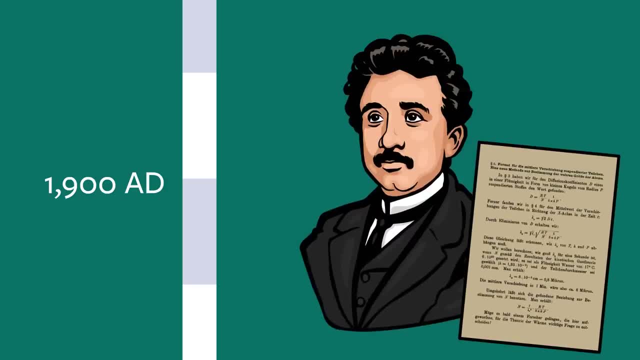 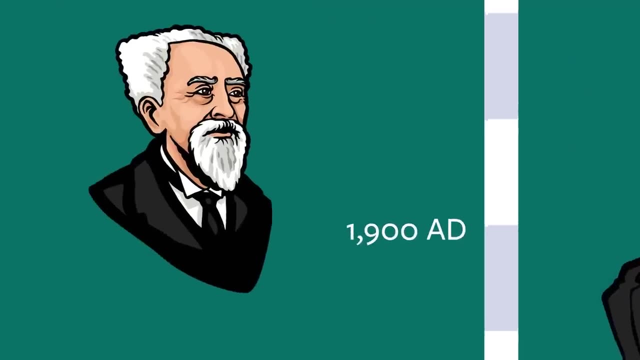 In 1905, Albert Einstein proposed an experiment and produced an equation that could be used not only to confirm the existence of atoms, but to determine exactly how big they are. A few years later, French physicist Jean Perrin- or I guess in French that would be something a little bit more common- 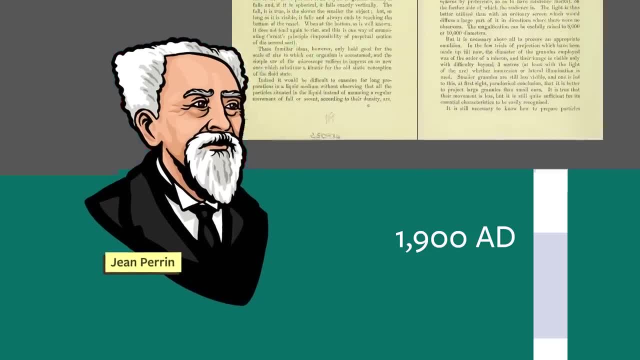 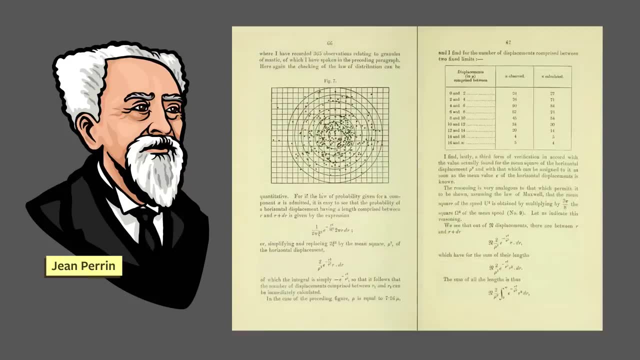 a little more like Jean Perrin, used Einstein's concept to actually do the experiments, confirming beyond reasonable doubt, at least to other physicists and mathematicians, that atoms do in fact exist. Now, if you happen to love math and possess an in-depth understanding of physics, 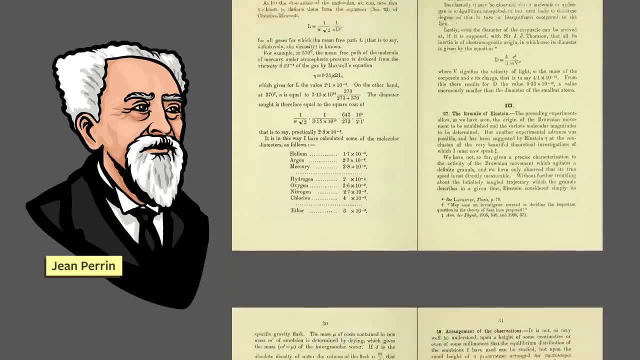 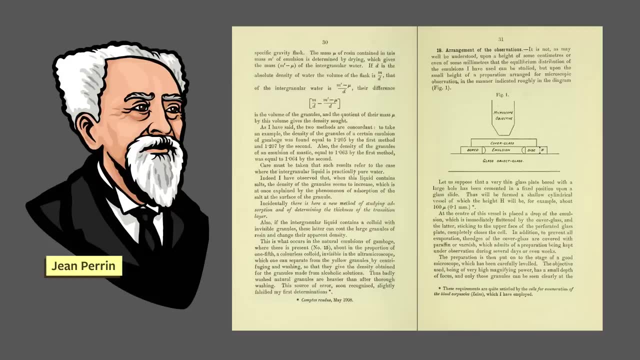 then great, You can just turn off this video right now and go read his book. But for the rest of us, a little visual confirmation that atoms actually do exist would be nice, right? Unfortunately, individual atoms are far too small to be seen with normal light. 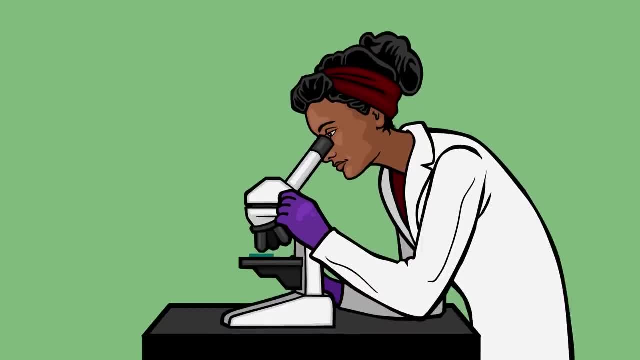 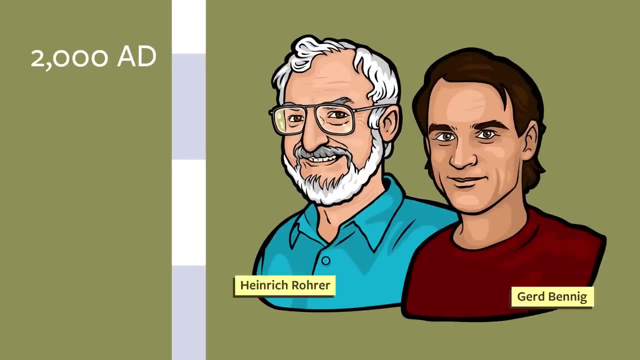 The wavelength of light is just too great. This means that normal microscopes cannot see atoms. In the 70s, a group of engineers led by Gerd Benig and Heinrich Rohrer began working on what they called the scanning tunneling microscope. 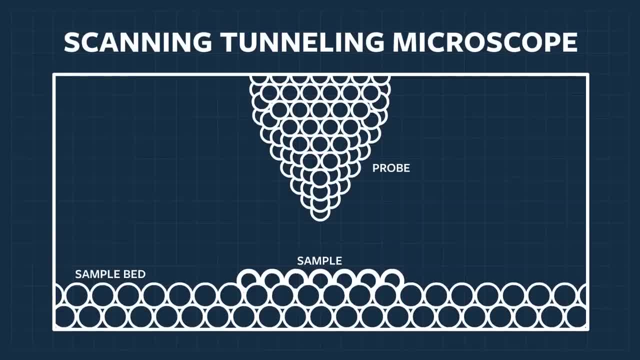 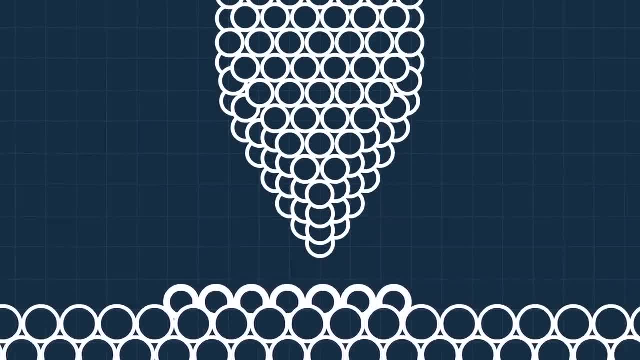 a microscope they hoped would let us take undistorted images of many different types of atoms. It uses a process called electron tunneling to scan and essentially feel the surface of the sample, much like you can feel around in the dark to get a picture of your surroundings. 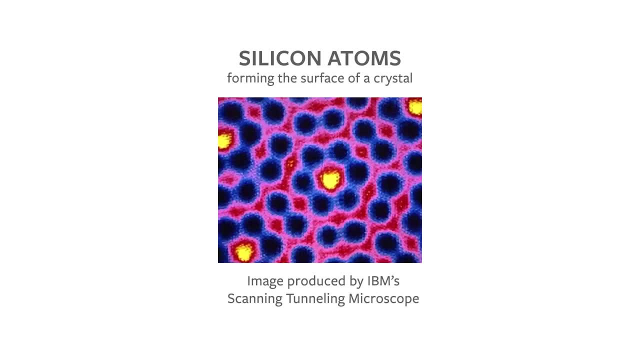 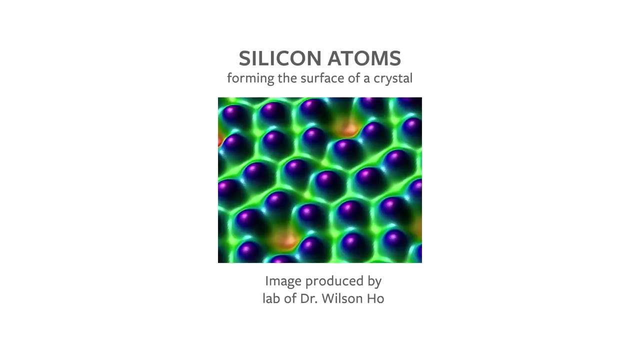 This is an actual scan of silicon atoms forming the surface of a crystal. The colors here are artificial, but this is real data showing the actual pattern of silicon atoms arranged in the sample. Later work by Dr Wilson Ho improved the technique and cleaned up the presentation of data. 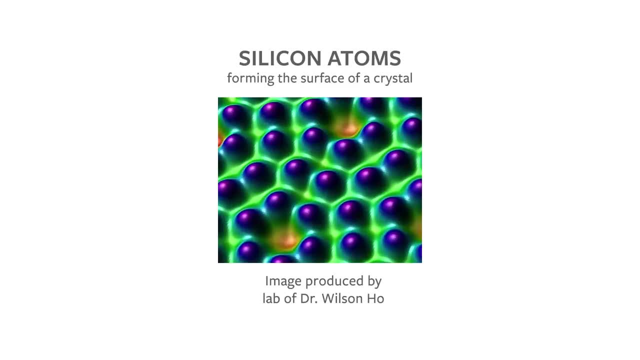 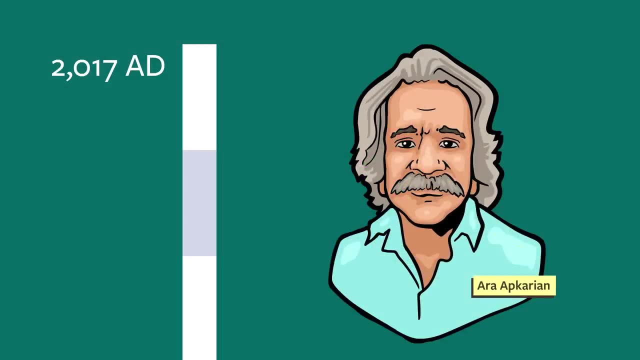 While quote feeling the atoms does give us good information, researchers still want to know what they are. They wanted more. A group led by Dr Ara Apkarian of the National Science Foundation's Castle Research Center discovered a way to use actual light to see atoms. 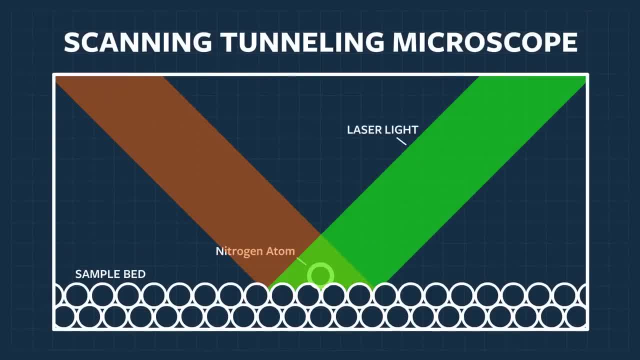 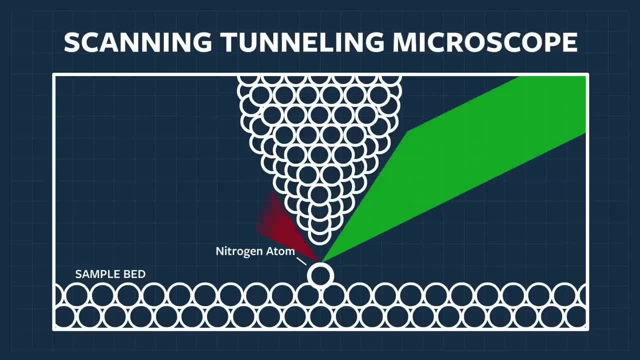 In the past this was thought to be impossible because the wavelength of light is so much larger than an atom. but by shooting light at the tip of a probe in a modified scanning tunneling microscope, they were able to essentially shrink the light's wavelength and get it to 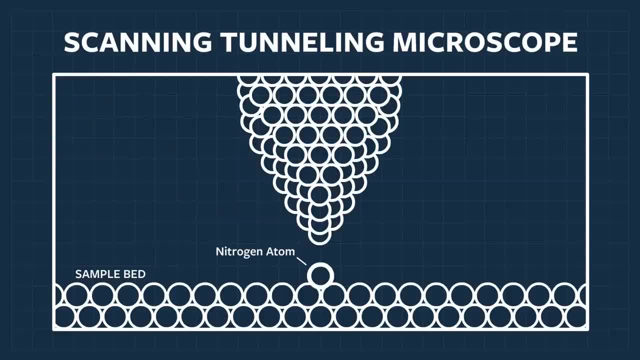 scatter off the sample onto a detection screen. By moving the sample bit by bit, the sample bit is now able to see the sample's wavelength. By moving the sample bit by bit, the sample bit is now able to see the sample's wavelength. 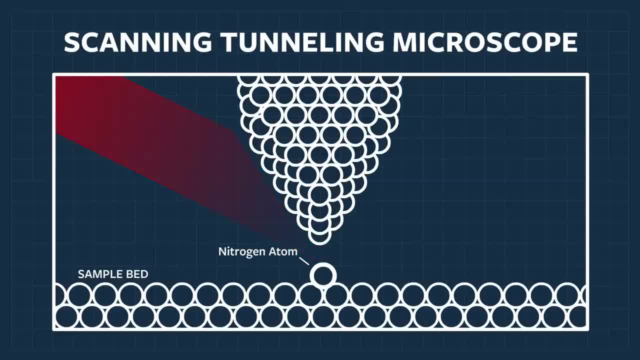 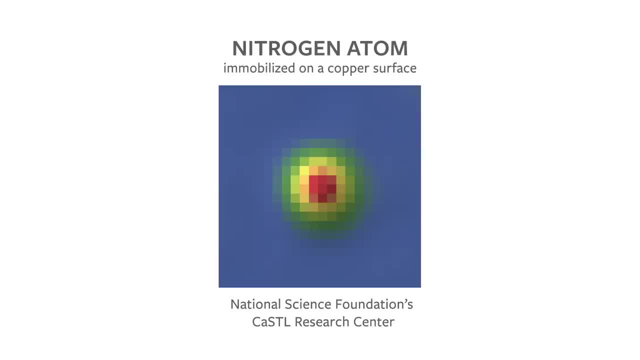 By moving the sample bit by bit. the sample bit is now able to see the sample's wavelength By hitting it with light again each time. they were able to piece together this image of a single nitrogen atom, each pixel representing an individual data point from the scan. 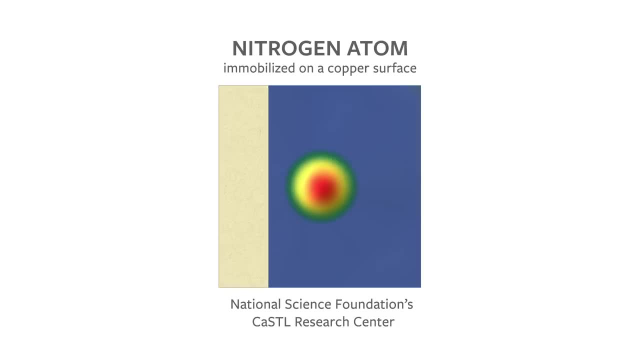 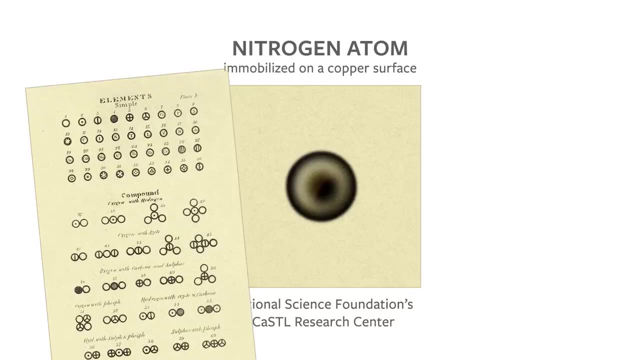 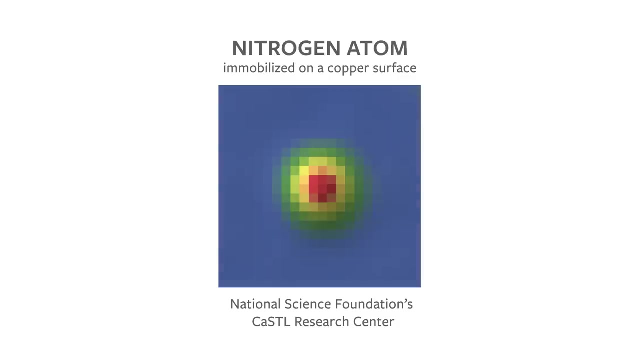 If we smooth it out, sharpen the edges and change their chosen color scheme. it is shocking to find how close John Dalton's old drawings actually were to reality. Our species has finally done it, Over 2,000 years after Democritus first proposed the idea of 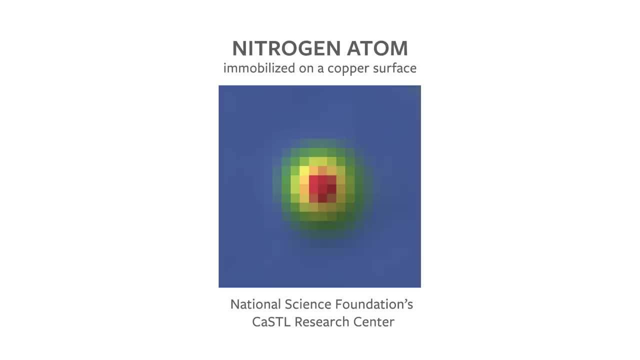 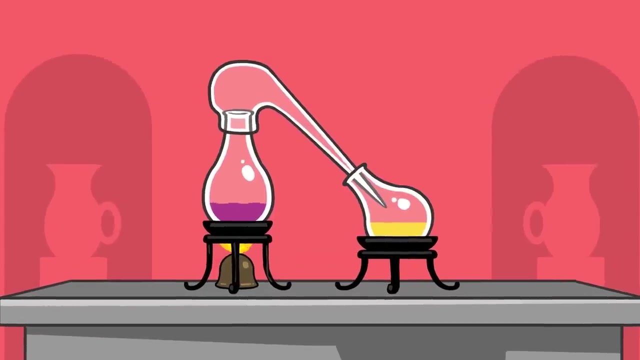 an atom. we have now received direct visual confirmation: Atoms exist. So, in summary, what is an atom? Atoms are the fundamental building blocks of chemistry. How do we know they exist? Through chemical reactions we can witness their effects. 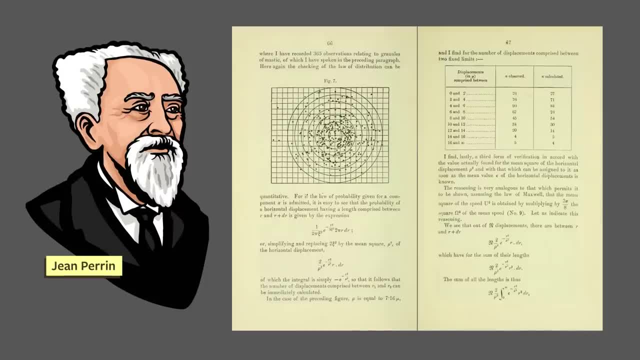 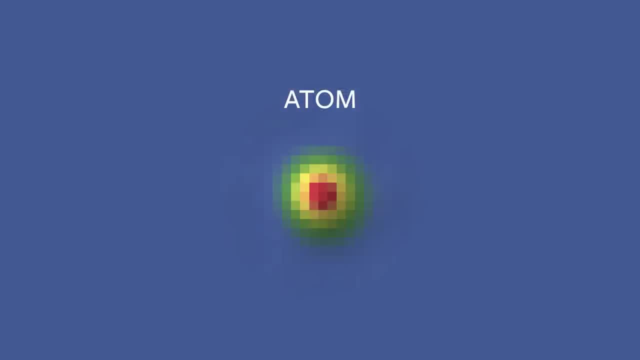 Through mathematical equations combined with indirect observations, we can calculate their various sizes. And finally, with the aid of new technologies such as the scanning tunneling microscope, atoms can now be seen. While the word atom technically means uncuttable, we'll see in the next animation that atoms actually can be split apart.